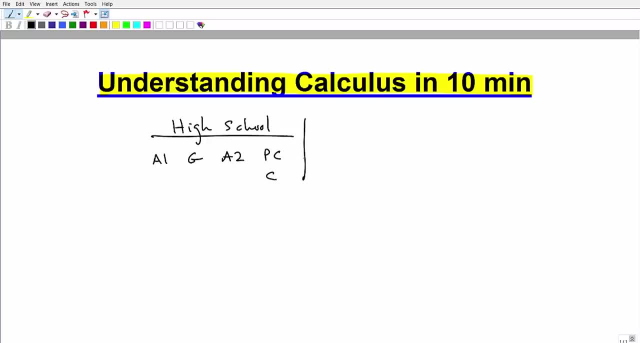 in their last year. Now, when you go to college, I would say maybe about 70% of the majors degrees in college. All right, So at the University level, many of them- well, definitely over half- are going to require you to at. 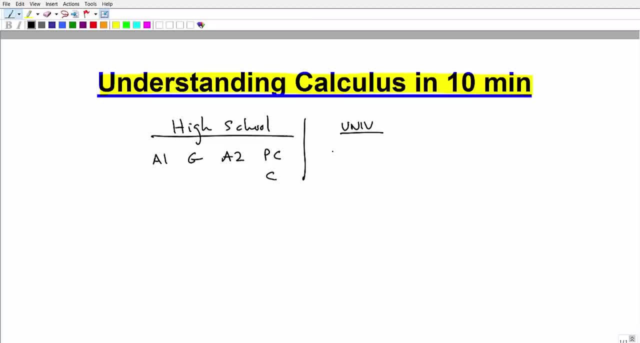 least have one semester calculus. so we don't take it in high school, you'll. you'll see a little bit of it in college. now, if you're some sort of science or technical major or finance or whatnot, you'll probably take even more of it. so 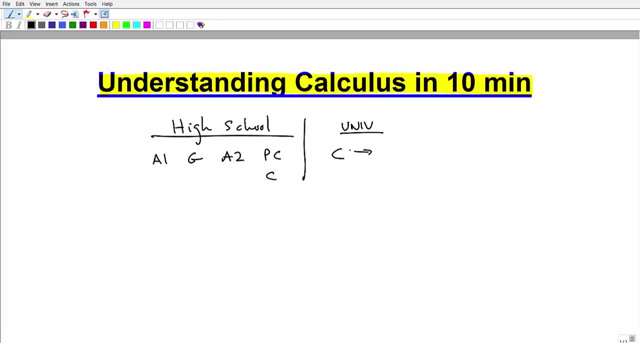 it's probably going to be, and a lot of your futures if you're going going the college route. okay, so that's just basically where where it lies in in the spectrum of learning. all right, calculus in 10 minutes, let's get right to it. so calculus basically helps us figure out kind of two problems, two kind of things. 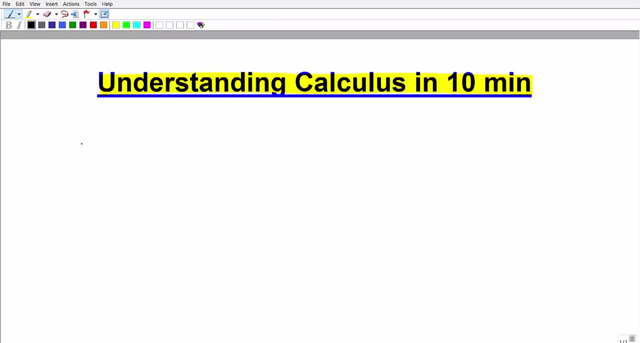 in math. I'm going to start with one that's kind of easy. that would be like the area and volume problem, okay, so I'm just gonna sketch out here real quick. you? so this is like a rectangle, right? so if I said, find the area of this rectangle, 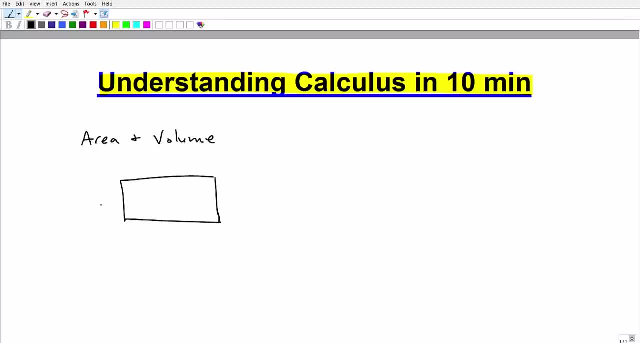 you. we have a formula for this, if you recall. so it would be like length times width, right? so the area of this rectangle is going to be the length times the width. no problem, okay, so we know this, because we were given a formula. let's do a circle, all right, what if we had a circle? and this is not a 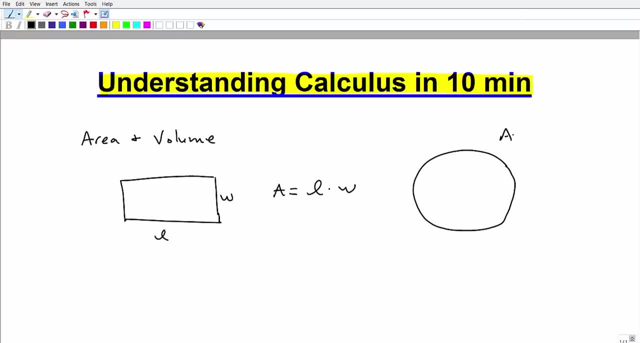 perfect circle, obviously, but if I said find the area of this circle, hopefully some of you out there, or maybe most of you remember there's a particular formula for this. okay, it's pi, R squared, R being the radius which is like from the center out this distance, and pi is a number of three. 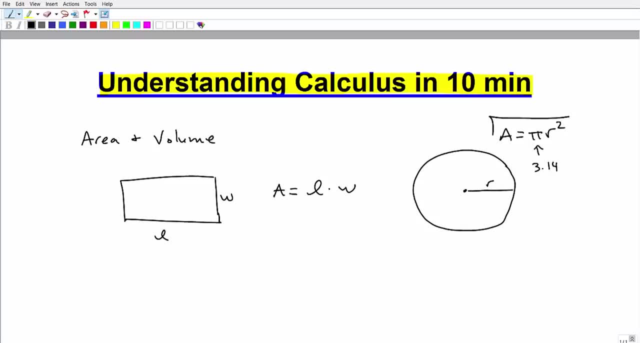 point one, four approximately. so I can use this formula to figure out the area of this circle. and for this rectangle I can use this formula. now let's just do one more example. what if I had a triangle? okay, so again, if I wanted to know the area, this would 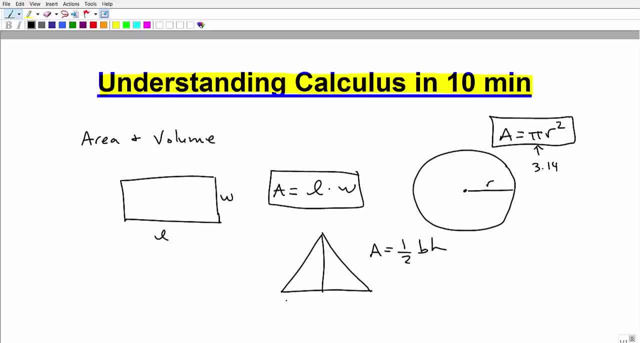 be one half base times height, right, so this would be the base of the triangle, this would be the height, okay, so formulas help us find the area and, by the way, this goes for volume as well. so these formulas come in handy with these kind of basic figures like triangles and, you know, circles and 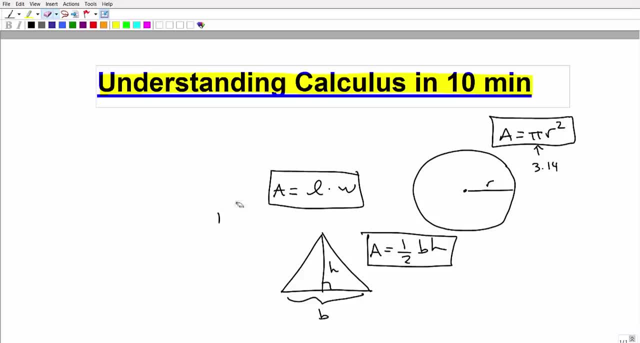 etc. so let's take a look at where calculus helps us out, okay, where it's a tremendous value. and, by the way, I can't overstate the importance of calculus and mathematics, engineering, science, I mean it's. it's huge really, is as powerful as you, you know, may think it is probably more so all right. so what if we had some? 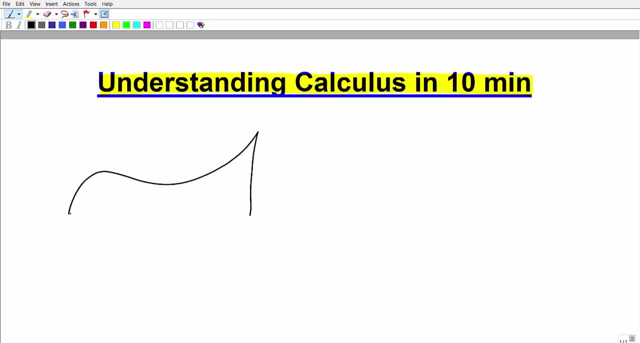 crazy figure like this, for example, and I'm just trying to draw something, you know may think it is probably more so, all right. so what if we had some crazy figure like this, for example, I'm just trying to draw something, okay. so what if I said: find the area of this particular object or this figure? 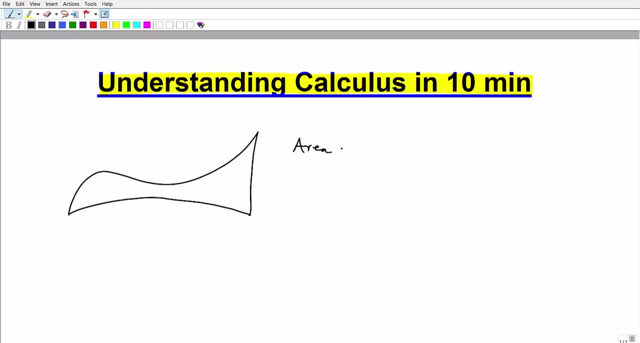 well, probably you're gonna be looking for a formula. right, you're gonna be okay. yeah, I could find the area of this. just give me the formula. well, guess what? there is no formula for something like this. this is very challenging, okay, so calculus helps us figure out the area of a crazy looking figures like this. okay, 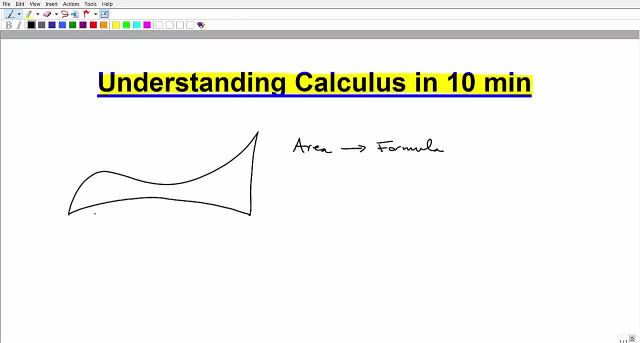 and volume. they don't have to be, as you know, you know, abstract as this, but but this is what calculus can do for us. this is the power of it, because without calculus we would have to go through and just kind of like maybe trying to estimate the area of this particular thing, but calculus can give us the exact 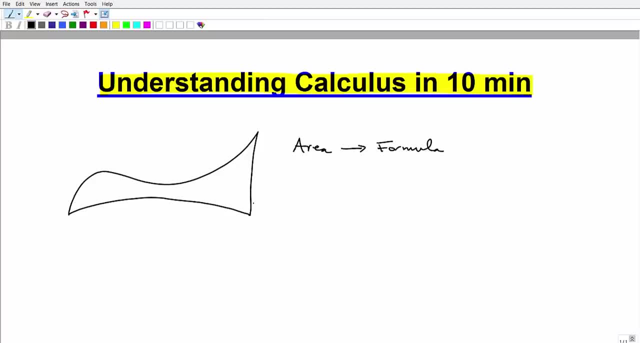 area. okay, now let's suppose that I took this, this figure, and let's let's kind of put this like on a, on an axis okay, and I circled it around, spun it around, so maybe it's kind of doing this business. I don't know what it would exactly look like, but it might look like. 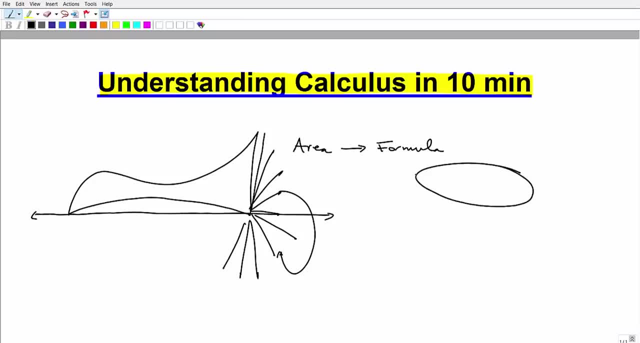 a, an object maybe, something like this kind of maybe sketching us out, all right, and then it looked like it would have some sort of hole in the middle, right, maybe like, like this type of deal very difficult to kind of maybe imagine, but let's try to figure this out, all right. okay, so if you did have this, it looks. 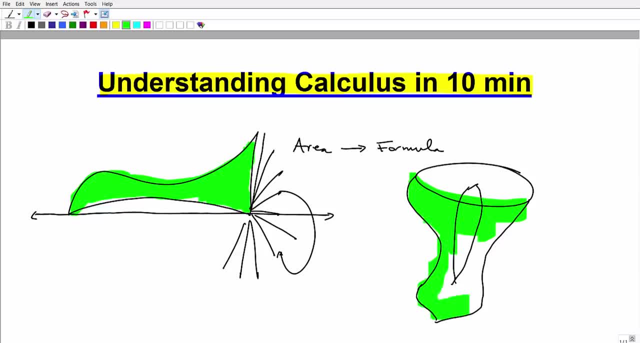 like this figure from some. we're looking figure: what if you did have this? okay, so maybe if you did have this, let's kind of fill this in a little bit, all right, and then you just kind of rotated this around, you would create some sort of weird looking figure like this: 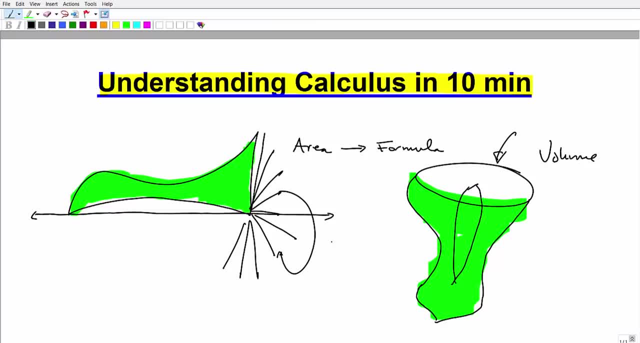 tell us exactly how to do this and You may think: wow, this is it must. you must have to go through all kinds of crazy Advanced calculations in order to do that and, Surprisingly, it's really not as bad as you think. Okay, once you understand the steps, you can do it. 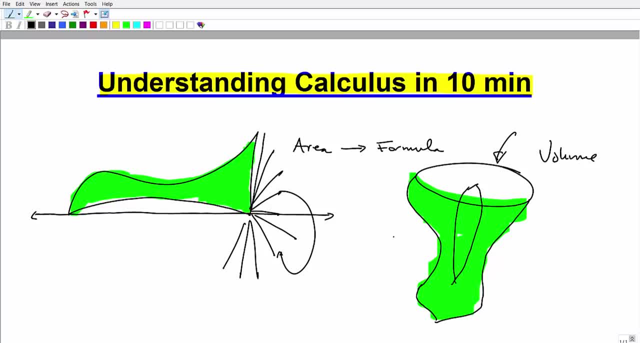 but you can see the power of being able to Figure this, this stuff out. Let's go ahead and take a quick look, a real basic example On how we will find area and volume in calculus. All right, so maybe some of you out there have already taken. 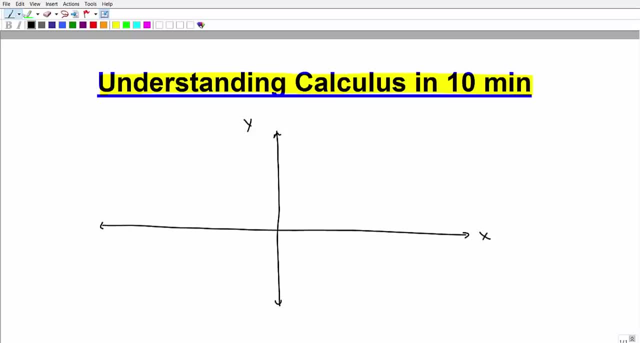 Algebra and whatnot. I'm just making a real quick XY axis. All right, let's kind of maybe Draw a little figure like so okay, All right. so let's suppose I wanted to find the area of From here to here underneath this curve. All right, let's say this area right here. 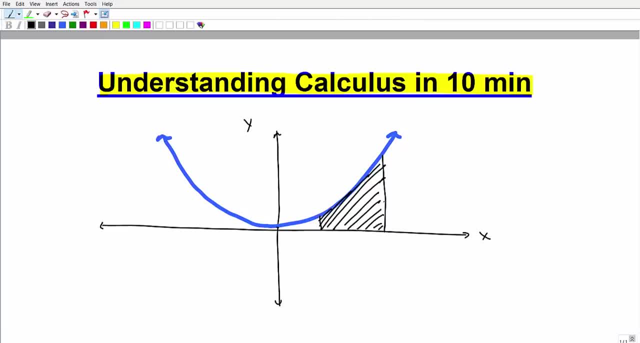 All right, let's say this Part underneath this curve. I wanted to find area so that that shape, if you look at it There's. it's kind of curves on top right it goes down. So you would be asked to find the area of This object. Okay, Once again, you're looking for formula. There is no formula that exists now in calculus or in mathematics in general. okay, 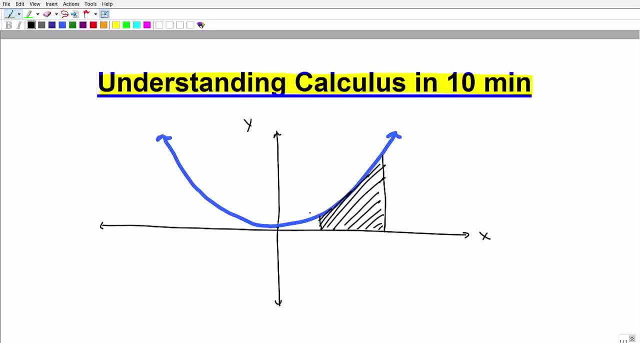 What we have When we have curves and things. we have little Things called functions, All right, they basically just describe the curve. So this curve Could be described by this: x squared. Okay, you don't really need to know that right now, because that's not the purpose of this video. 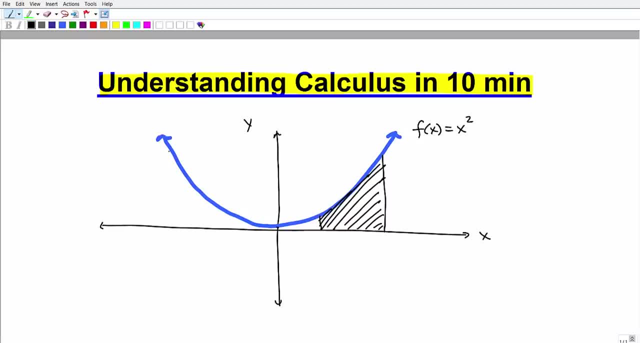 But this, this little rule right here, just just describes this curve. This is the rule that tells us that this is The. the shape of this is described with this particular rule. Okay, we call these things functions. So as long as you have this, This function, or the description of what of this, 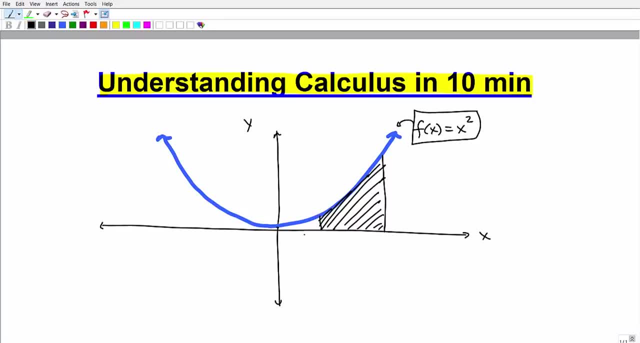 Curve. okay, then we can use calculus to find the area. so let's say on our little graph, This is, let's say, one, this is two, Let's say this is three, four and five. okay, so what? the way we would do this is we would go ahead and and. 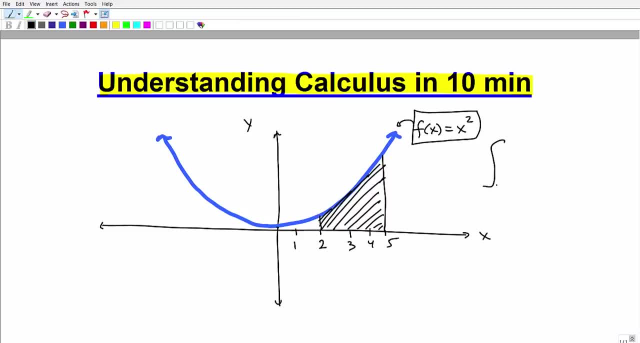 Have this little crazy symbol. Okay, you might've seen this this before. it's called the elongated s, but it basically means the sum. okay, and I don't want to get too far into it because that's not the purpose of this video, but we're going to say is, hey, we? 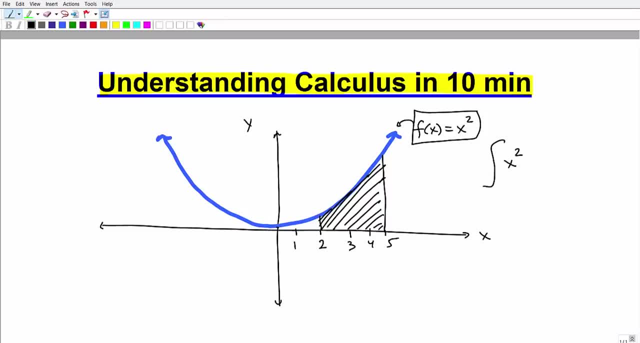 want to find the area underneath this particular curve and and I want you to start from two and go to five. all right, so that's how we write that. okay, then we put a little tiny little dx here. that will be kind of like in my part two of this video here. I'm going to get to that in a second. 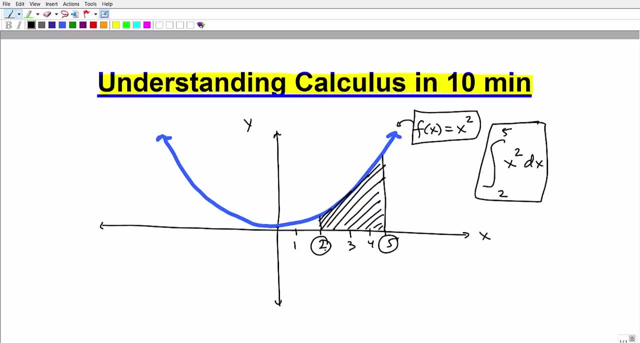 okay, but but this is the setup. all right, to find the area underneath this curve. okay, you're saying, well, yeah, that looks pretty complicated, that's fine, but really, and and the the steps to actually find the area are not complex at all. what we do in calculus, once we write this out this long thing, 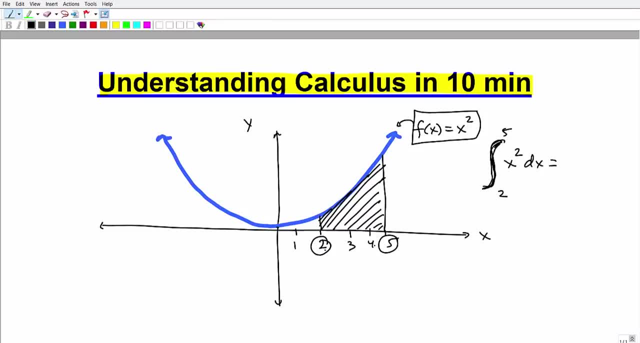 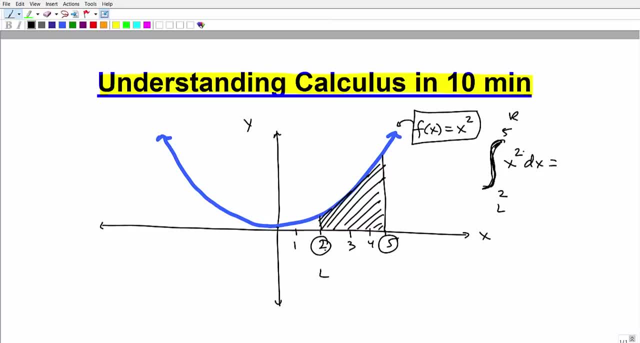 side of the curve, and this is to the right side. not difficult, right? this is the description of the curve. once again, if we're given it, not difficult, okay. so what we do now okay is there's a little rule that says: take this number, this exponent in this power, you just add one to it. 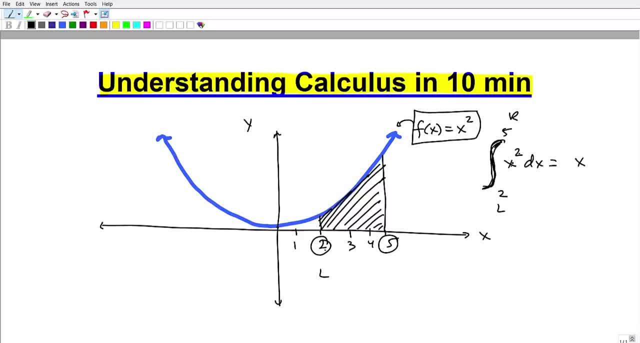 okay, so we're going to keep that same variable. add one. so two plus one is what? three? pretty simple, then, whatever that result is, we're going to divide by that number. okay, so all we're going to do is take this right here and we're going to use this to find the area. the way we do that is the following: 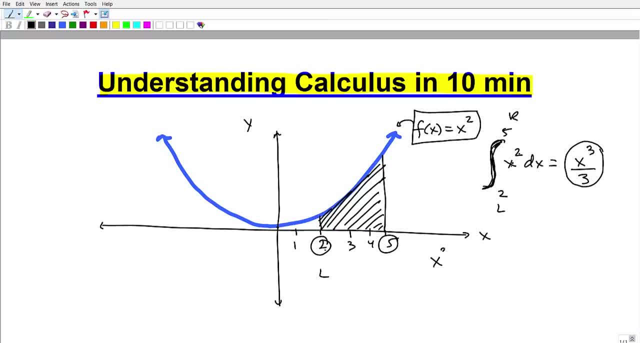 okay, we're going to subtract. we're going to use this thing, all right, and we're going to subtract the following: okay, we're going to plug in five over here. okay, we're going to start from the bigger side, so we'll plug in five cubed right from our right side, and I'm not going to get too far into it. then we're. 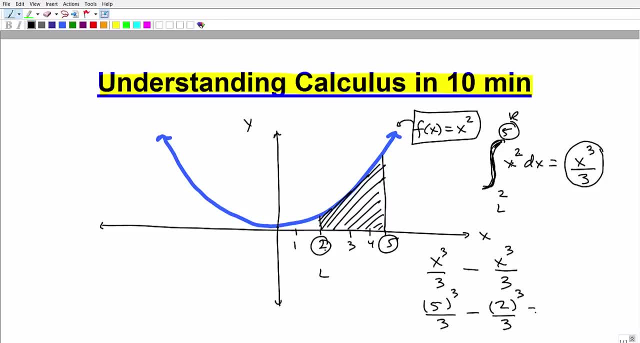 going to plug in from the left side, like so, and when we do this little calculation, okay, we're going to actually get the area. so it's really not difficult in terms of the- uh, you know a mathematics involved. I mean, if you take in basic, maybe even pre-algebra- you know middle school math- you could. 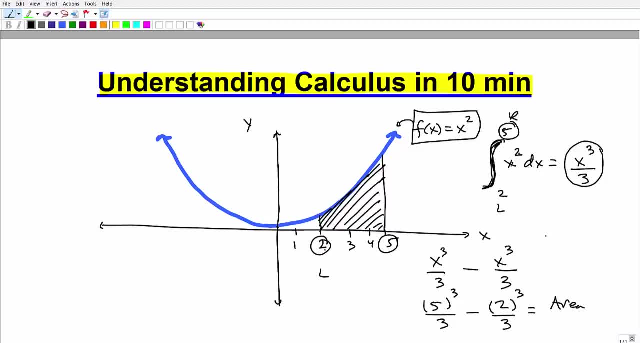 figure this out right. I would just, obviously I'm telling you the steps now. what gets calculus, what makes calculus more complicated for people, is that these curved descriptions, these little um curves and these functions. they you can get more complicated. okay, so when these get more complicated, you have to learn more rules. but it's really a matter of just learning the rules to to. 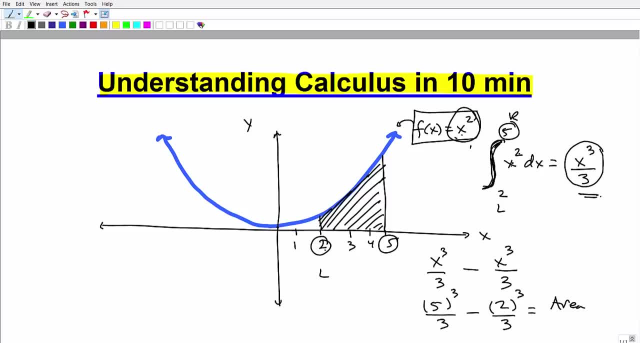 get to this part. okay, so that's the big deal. this is like part one of uh, of calculus. okay, now calculus, like I said, there's like two big problems it solves for us. so that's the first problem area and volume. let me erase this and then we'll get into the second. cool problem. all right. 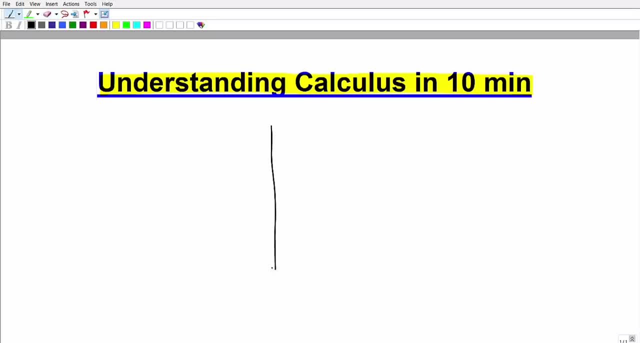 right. so the second thing calculus does for us- and let me go ahead and draw a little x, y plot- here is: calculus helps us determine how steep okay something is, what its slope is, all right. and what do I mean by this? um, let's suppose, from here to here, I wanted to know generally how steep this line is going. 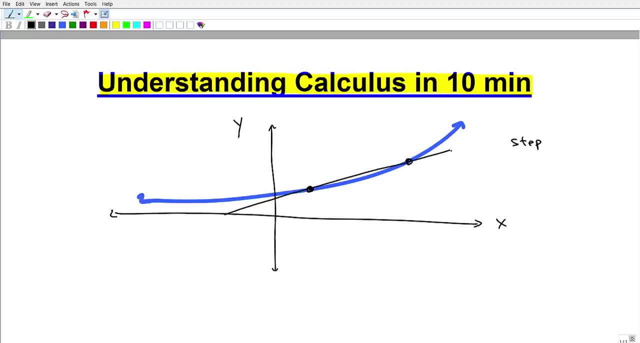 from these two points. so I could say, well, it's kind of going this direction. now I'll get into why this is important here in a second. we want to know the, the direction of curves. okay, we want to be able to get their steepness, because they're always changing, if you. 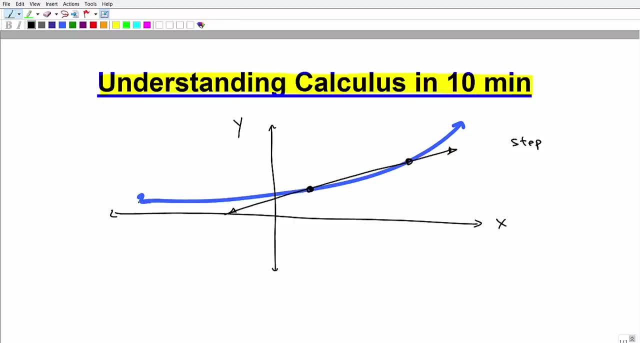 study this curve. this curve is always changing. this could be, for example- just imagine this can be anything you want it to be. it could be population growth right over time. all right, if you go to your consumption, you do the math and come up with the handle here. this is the. 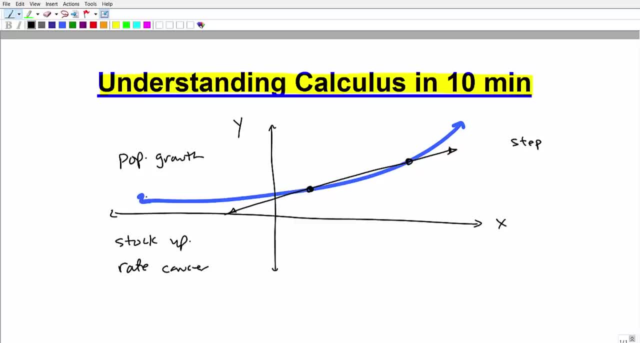 primer at the top of hours after hours. so if you intersect the two Kentucky numbers, you actually get defense. you can say, okay, I've broken this up, it's this is because I've been singing all this time. so check and out if it is that's good or if not. it doesn't matter, because that's if it is necessary, if it's. 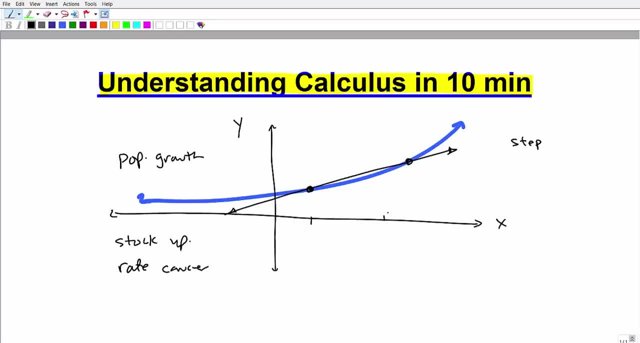 it's or or between blocks of the curve. it's the steepness. okay, because this gives us an indication of where things are going. you could tell here: the steepness is different here versus where, let's say, at this point in this particular graph. okay, so the steepness is always changing. all right, we call. 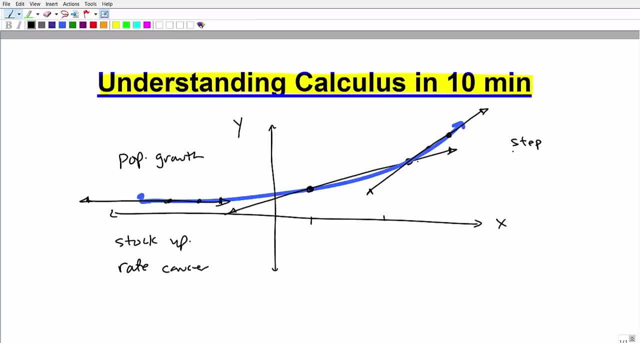 this. we call this steepness. I kind of like to use the word and I'm using step, but it's really a steepness. okay, there, my word is, but actually the technical word is slope. all right, that's probably better for you anyways. so it's the slope. 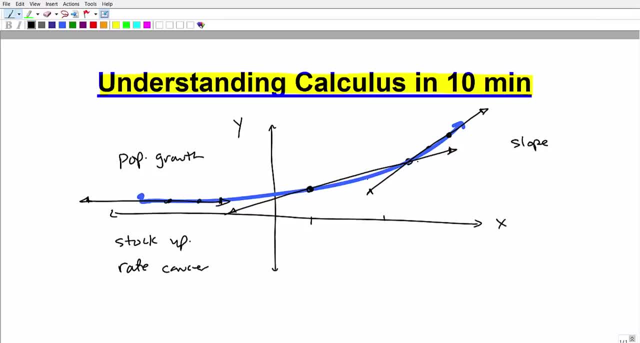 of the curve like hey, you know how, where is it kind of? so what's its actual slope? now you can figure out the slope. if you have two points are on the curve, it's pretty easy okay, because effectively what you're gonna do is just determine, like this, these two points, I can just figure. 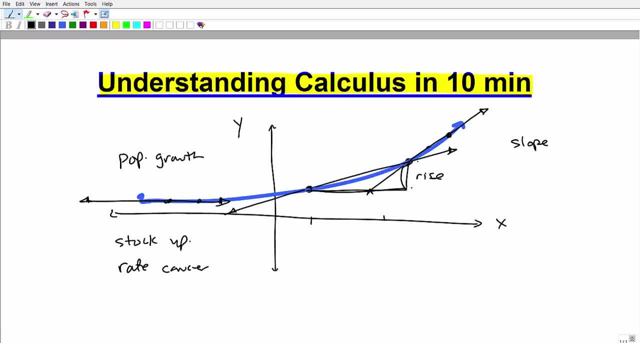 out the rise, and that's just this amount right here over the run. okay, so the slope is defined by the rise over the run. so if i can get those two measurements, it's no big deal. i can just figure it out and there there i go. but here's, here's where um calculus really becomes powerful, okay. 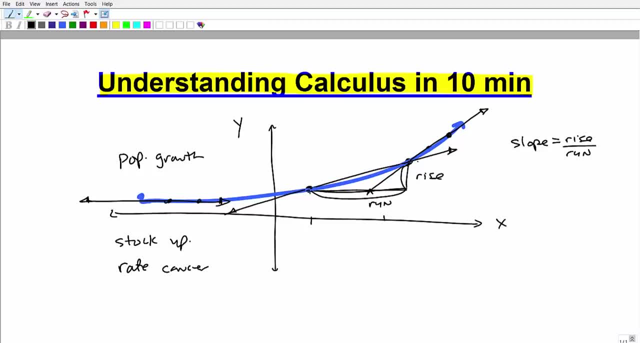 what happens when we want to know the slope of a curve. and let me just- i'm going to draw a new curve here to make this a bit more pronounced- okay, maybe something like this: okay, so we can see that the slope here is kind of going, it's kind of doing this, and then it's kind of like: 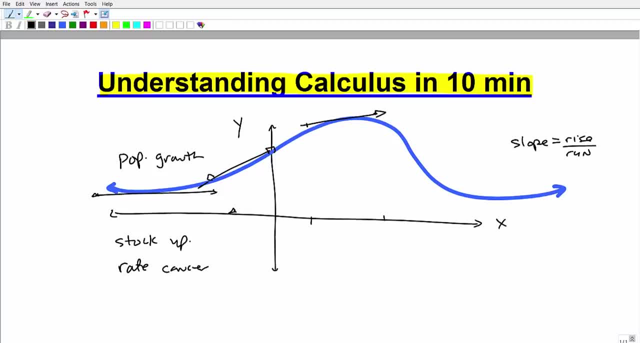 going this way. then it's kind of going this way and then it's going down like so right, so the slope of this curve is constantly changing. now, what if i want to know the exact slope of this curve at this point, right here? okay, that point. well, the by definition, the slope we need, the rise and run we actually 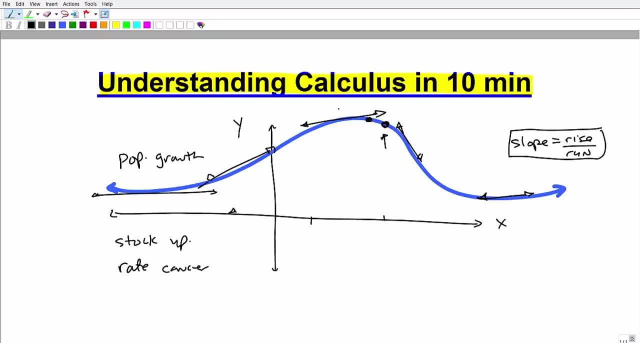 need two points like here. i can kind of estimate it right. if i take two points, it's kind of going in this direction, okay, kind of something like that. but if you notice, if i put another point right here, it's kind of going like this. so you know, i'm getting different. 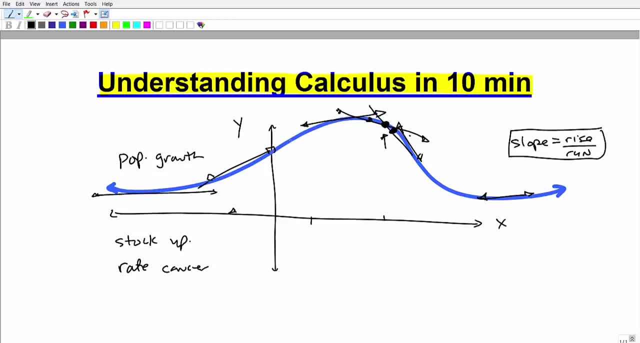 things. i'm getting different things. i'm getting different things. so what i want to do is i want to estimate. i want to know the exact slope right on one point of a curve. okay, and you can think of this as as the exact rate of change in one precise moment. all right, so let's think of this as time. 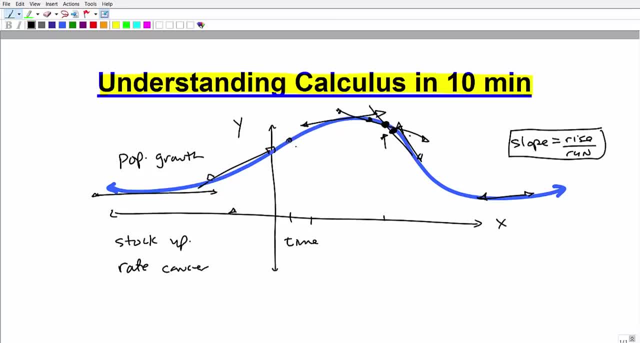 okay, and maybe this is population growth. i want to know the exact rate of population at this exact time. maybe it's, uh, may 8th of whatever year. okay, at what particular time you want to know exactly. you don't want to know. an estimate kind of goes back to our area of my palm. you can get estimates. 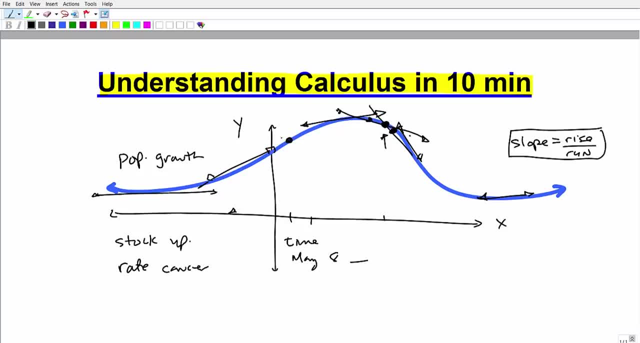 but not the exact answer. well, calculus helps us determine the exact, exact answer, because in calculus we can determine the slope. now, once again, what we need is the function. okay, let's say- and this for those of you out there, this is not an actual, um, the actual function to this curve i'm 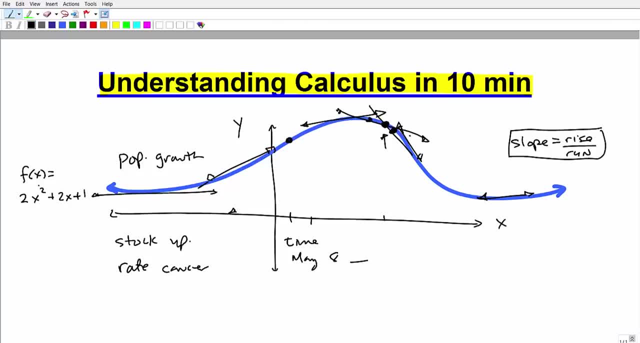 just using this for for simplicity stakes. but let's say i had this function described by this uh rule. okay, now remember, we use these function descriptions as uh, uh when we're trying to find an area of volume in calculus. but here we have something called a derivative. all right, and the derivative basically is it's. 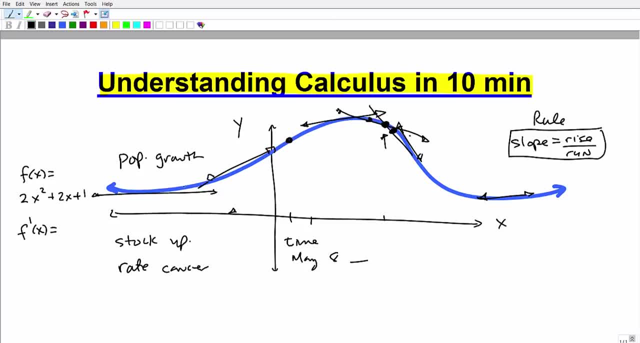 uh, a rule, okay, that allows us to find the slope at any point, at any exact point along the curve, and that's what that symbol looks like. this it's also looks like. so, all right, this is another symbol in calculus: DX over dy. and there's even other ones: f, prime, etc. but these crazy symbols are: 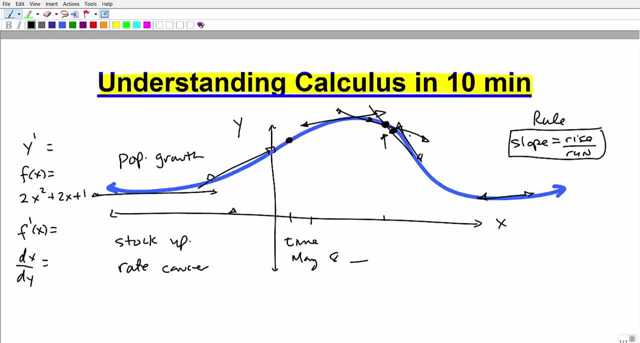 the derivatives. so let's take a look how I would find the derivative of a function of 2x squared plus 2x plus 1. all right, so what we call? we call this actually the first derivative. so all we do is we multiply this exponent 2 times. 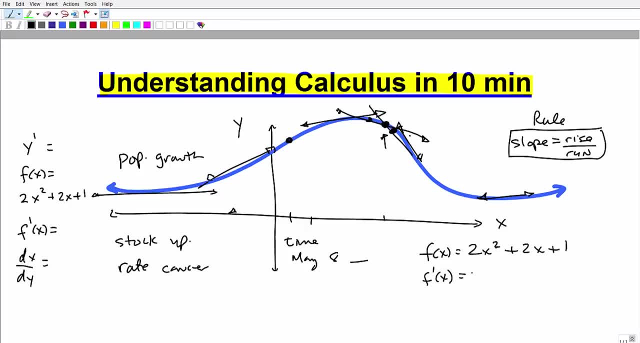 this coefficient, this number. so 2 times 2 is what 4? we keep the X and then we subtract 1 from this 2, so that's just X to the first one, or just X. now we go to the next guy and we do the same thing. so this X, here there's actually a little 1. 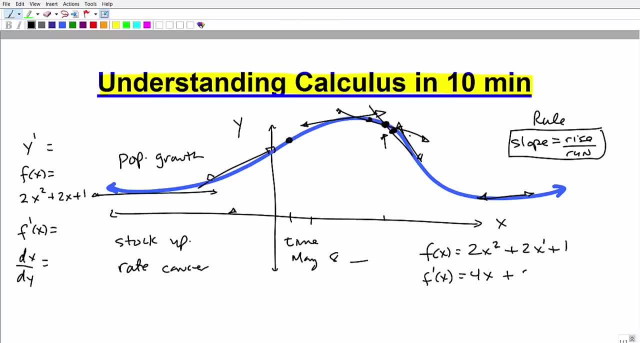 we don't write it, but there's a 1 up there, so 1 times 2 is 2, and then X here to the 0, so that's gonna be just X to the 0. power is just 1, so this is our first. 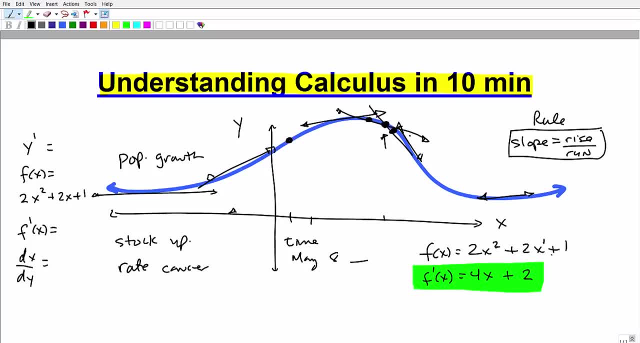 first. second, a derivative, okay, of this particular function, this curve description, and this is a rule to tell us the slope of the curve anywhere along the curve. okay, but you can see here the what I just did. the mechanics of finding this are really quite easy. once again, it's a bunch of rules, so I can use this. I'm not gonna. 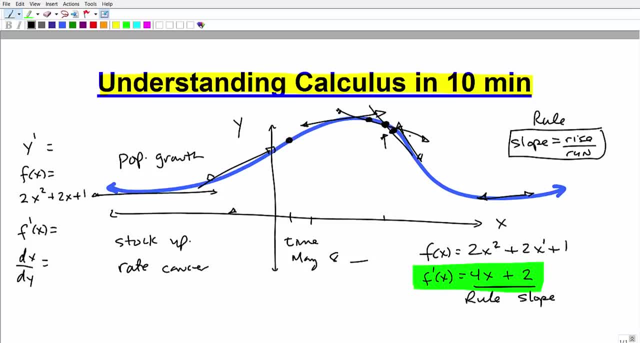 get into this now, but I can use this here, this particular rule, to easily find the, the precise slope at this moment in time. okay, and this helps us solve tremendous problems in mathematics. okay, here let me, let's, let's kind of, maybe kind of, first of all, let me kind of clean this graph up. let's say you wanted, 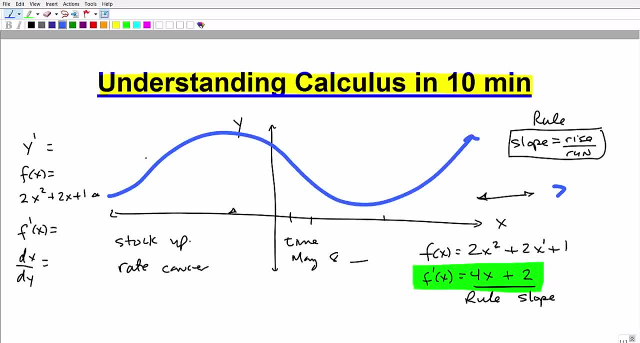 to know, let's say, we're doing some sort of scientific study- actually we do the better curve- and let's- let's suppose this is maybe some sort of medicine or pharmaceutical drug that you're testing, okay, and you want to know like, hey, wow, this is where it's decreasing. you know the symptoms of 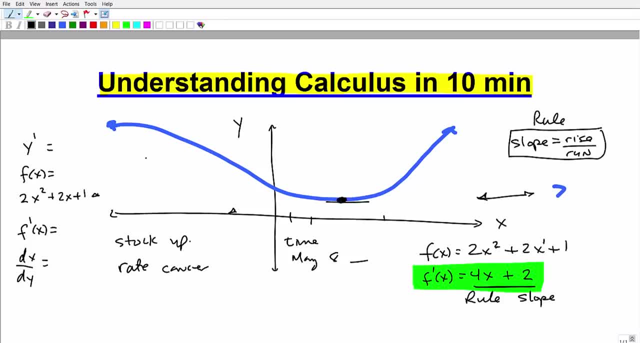 you know, let's say cancer, you know, or reducing, you know, bad blood cells in your body or whatnot. you know here, you know you're testing, your testing, your test, and you want to know, wow, this curve is telling me right in this area at this, to say dosage okay, or or combination of what you're using is what works the best. 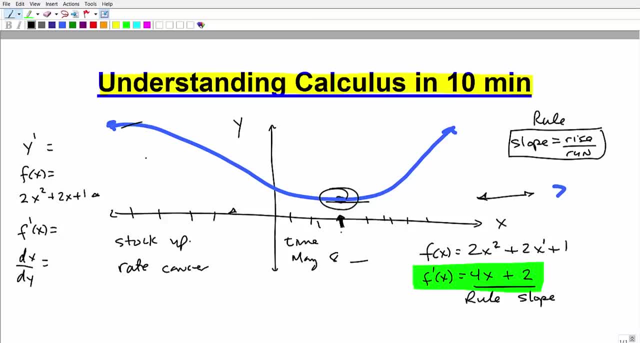 and minimizes the issue. so you want to know exactly what this point? okay, so you wouldn't want by finding the slope of the curve right here. this is what allows us to answer these things precisely. okay, they're called like maximum and minimum problems. so, anyways, I'm sure this video went over ten minutes, but hopefully you. 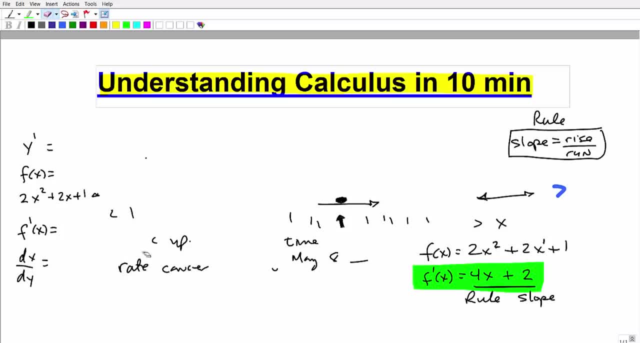 got something out of it right. this is the big deal with calculus. it is a big deal. it's a huge deal, okay, but it's not. it's not impossible to learn, even if you don't have a math background where you're, like, super strong in math and you. 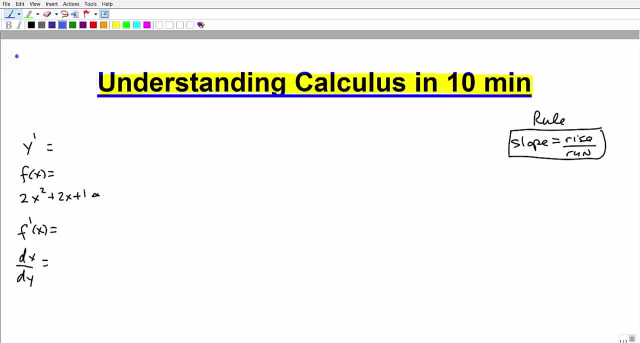 struggled math, you can get through calculus, all right. you could definitely get through calculus, but it does require you to study a lot of rules, and you know. the best way to get through calculus is you get through calculus, and you need to way to approach it, though, is to understand the value of calculus, so remember the two big things. 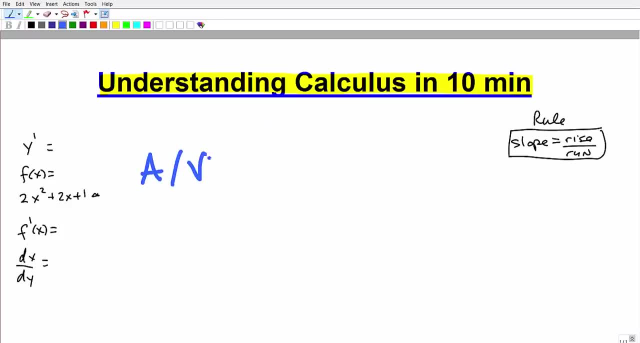 that we study calculus for is to help us with these area and volume problems. that's huge. okay, we use the integral for that, all right. and then the other thing is to um is to find the slope. okay, call this the derivative. so we use this symbol, okay, all right. or this symbol: y prime. 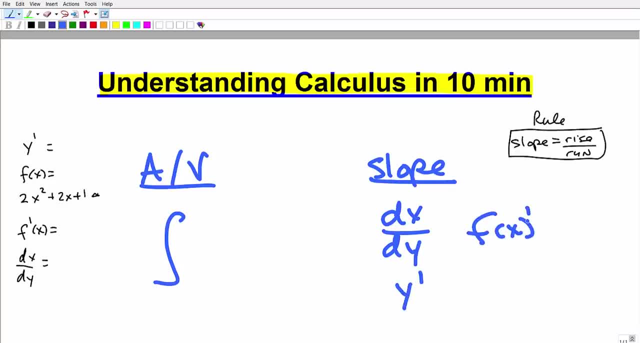 or this symbol. there's multiple symbols. they mean the same thing. okay, all right, so hopefully you got something out of this video. um, for those of you out there taking calculus know a lot about this. uh, and you're saying, oh well, this is not technically correct, or this and that. well, listen.